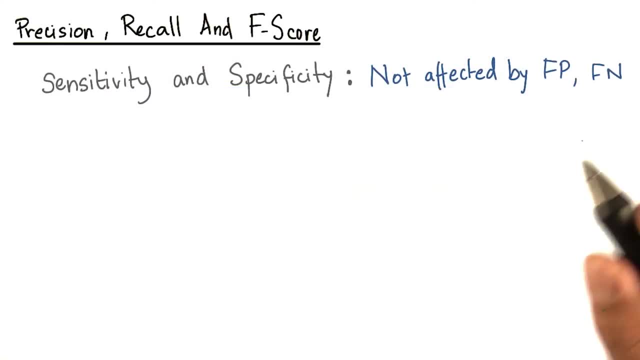 to the precision, recall and F score video 28.. The sensitivity and specificity of a classifier are symmetric measurements in the sense that the changes in false positives or false negatives do not affect the sensitivity or specificity respectively. Thus, in our example, we had two instances of classes B and 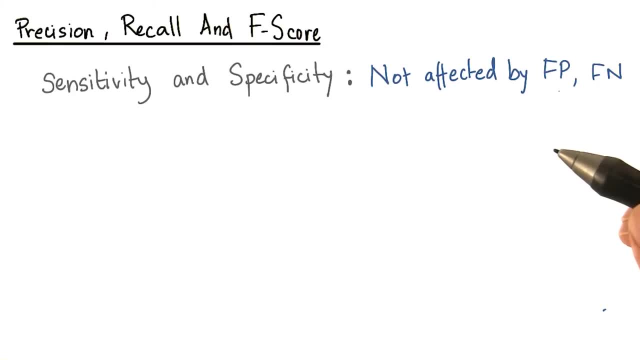 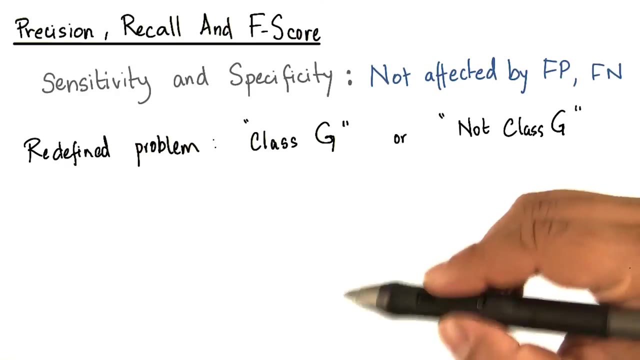 F, And we decided thus: in our example we had two classes, B and F, and we classified between those two. Now we re-ask the question to see if we can choose between two classes that are asymmetric. In our new problem we have 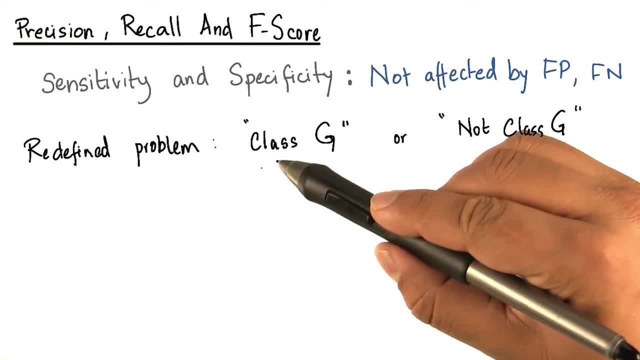 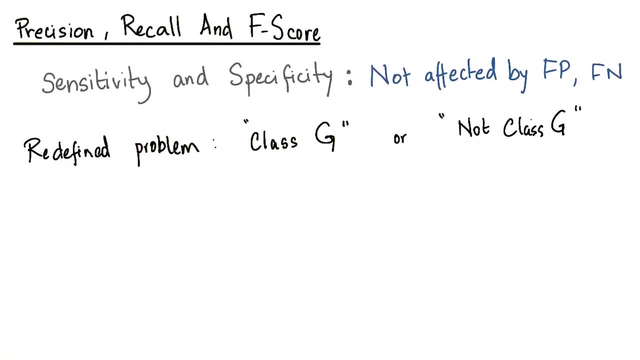 slightly redefined the problem. We want to ask if something belongs to class G or not class G. This is a one versus all classifier. We're going to look at some metrics called precision, recall and F score. that helps us in validating classification problems and models based on these kind of classifiers. 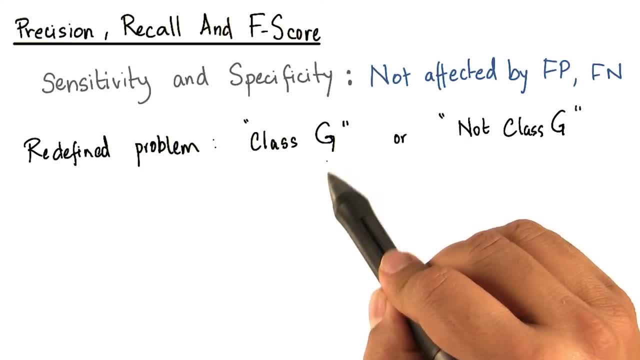 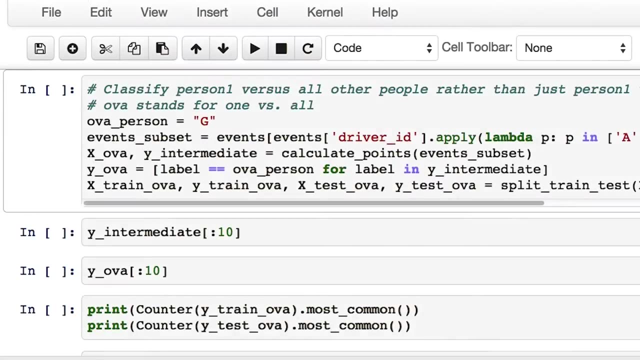 The difference being the instances for class G are a lot less than the instances for not class G in the data. Let's get back to our IPython notebook and see how we can build these models. first, In this piece of code, we are starting to classify person 1 versus all. 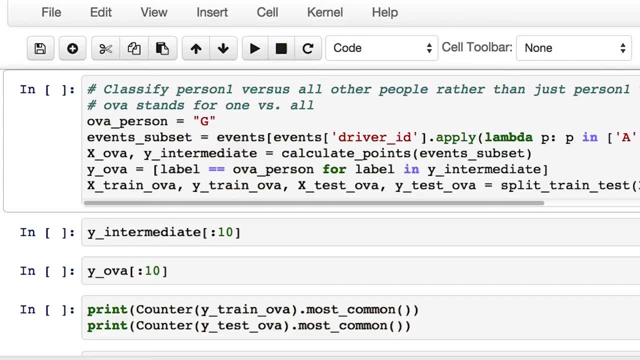 We call that OVAperson or 1 versus all person, And we choose G as that class. We now divide up the events such that we have G and not G as the two classes. Let's run this piece of code first. In the previous piece of code we have set up the. 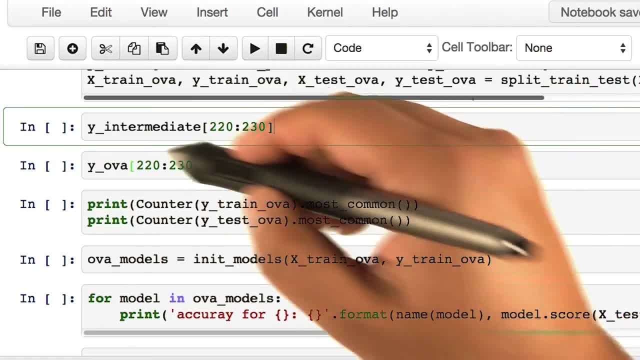 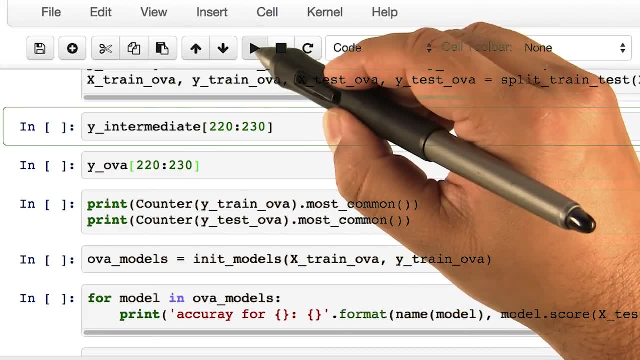 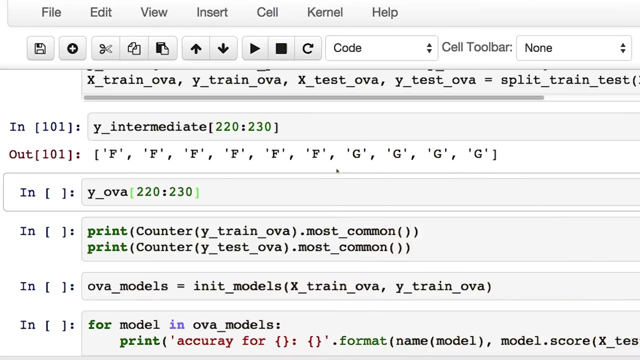 versus all data. Let's look at what the y values are between the indices 220 to 230.. Run this piece of code now. You see the ten values are f's and g's, with the last four values being g. Now let's see how this looks when we have the one.